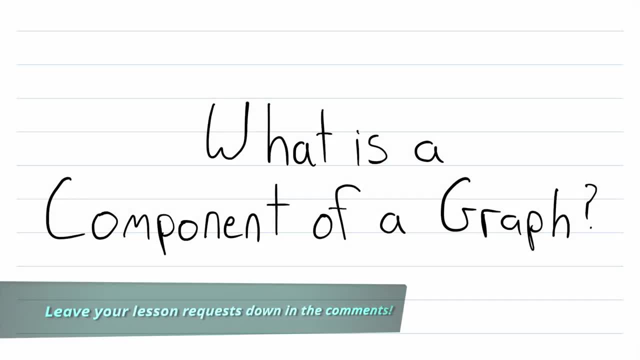 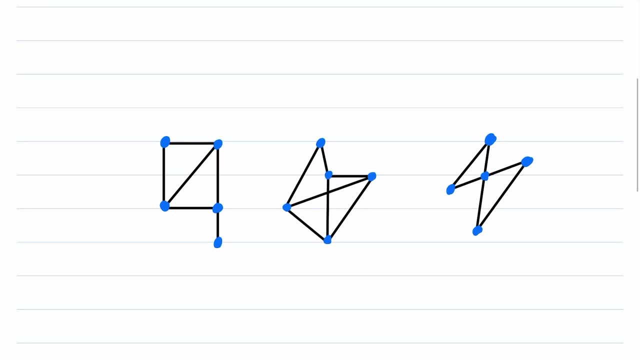 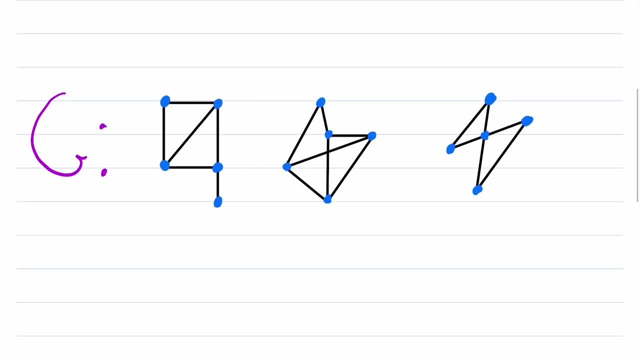 Hey everyone, welcome back to wrath of math. In today's video, we'll be answering the question: what is a component of a graph? shouldn't take all too long, So let's get right into the lesson. This is the graph we'll be using for this lesson and we will call it G And our beautiful graph G. 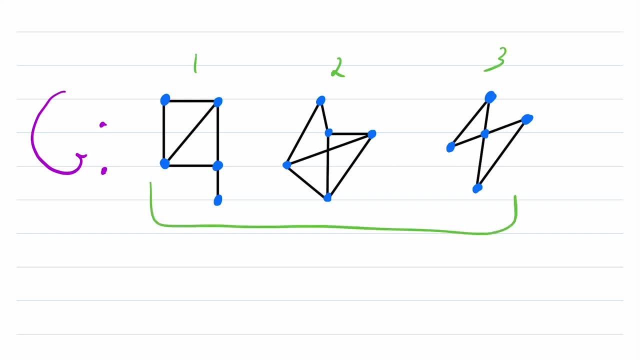 has 123 components. a component of a graph is a maximal connected sub graph. So what does this mean? Well, let's take a closer look at our example in order to find out. This is a component of G. But why is it a component? Well, for starters, it's quite clearly a sub graph of G. 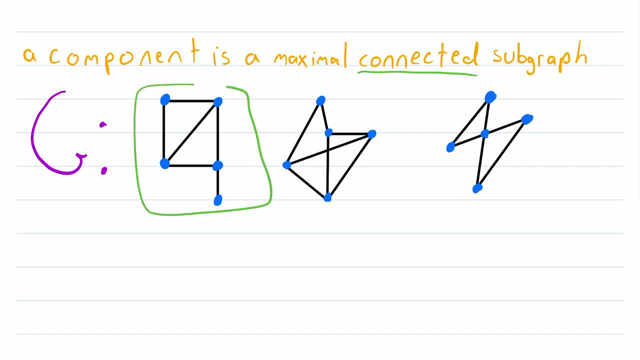 we can also see quite easily that this sub graph is connected. It's connected because there exists a path between every pair of vertices in this sub graph. From any one vertex you can get to any other. So it's a component of G. And what does this mean? Well, let's take a closer look at our 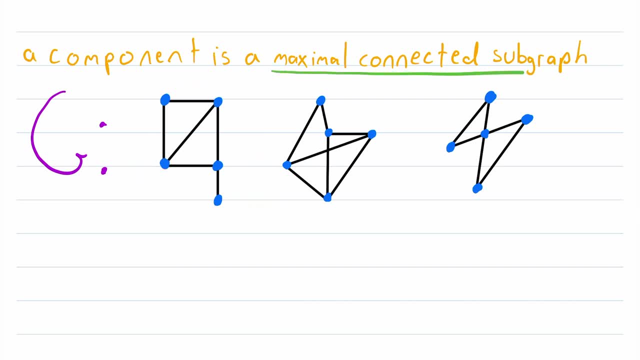 example, in order to find out. This is a component of G. But why is it a component? Well, for starters, it is a connected sub graph. then what makes it a maximal? connected sub graph? Well, maximal can mean a couple different things, depending on the context, But in this case, we're talking about this sub. 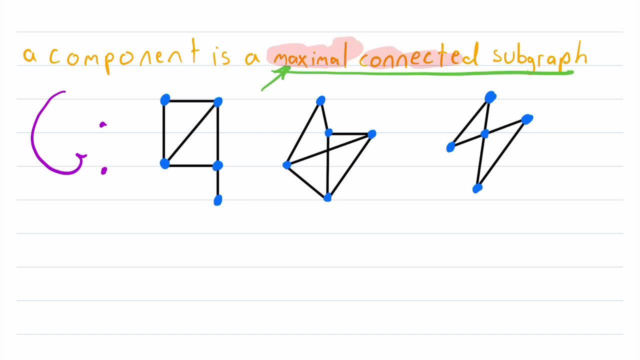 graph being maximal with respect to connectivity, And what it means is that we cannot extend this sub graph by adding in any combinations of vertices and or edges while preserving its connectivity. There is no combination of vertices and or edges while preserving its connectivity In the graph G that we could add to this sub graph and still have a connected sub graph. So 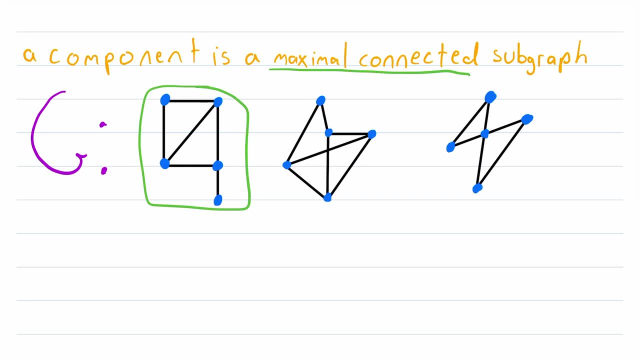 that's why it is called a maximal connected sub graph And to try to make that more clear, let's look at an example of a connected sub graph that is not maximal. we could look at these four vertices and four edges. This is certainly a connected sub graph of G, but it is not a maximal. 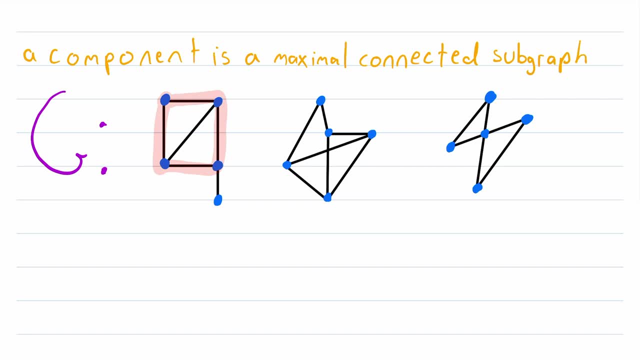 connected sub graph And so that's why it is called a maximal connected sub graph. But it is a connected sub graph Because, for example, we could extend it by adding in this edge and we would still have a connected sub graph. Even if we added that edge, it would still not. 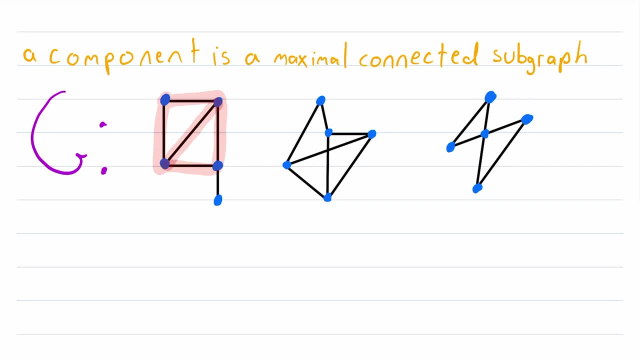 be a maximal connected sub graph, Because of course, we could then also add this edge and vertex. But now this whole thing is a maximal connected sub graph. there are no vertices or edges that we could add to this sub graph while preserving its connectedness. Therefore, it is a. 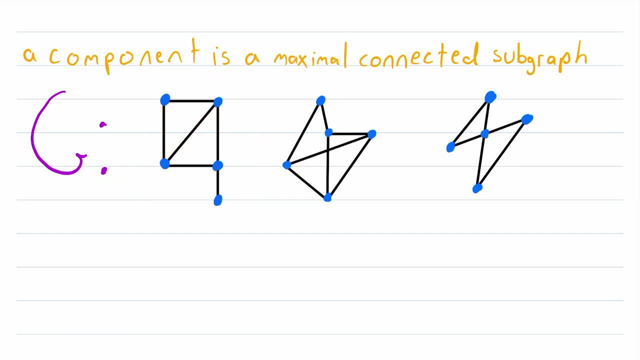 component of the graph G. For another example, we could look at this sub graph of five vertices and five edges. This is a connected sub graph, but it's not a maximal connected sub graph, Because we could extend it while preserving its connectedness by including this edge, If we were. 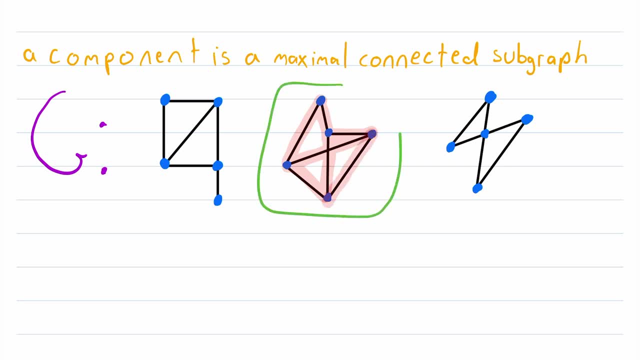 to include that edge. then we would have a maximal connected sub graph And therefore this is a component of G, there's a component of G. there's a component of G and there's a component of G. There's no combination of vertices or edges that we could use to extend the sub graph, while 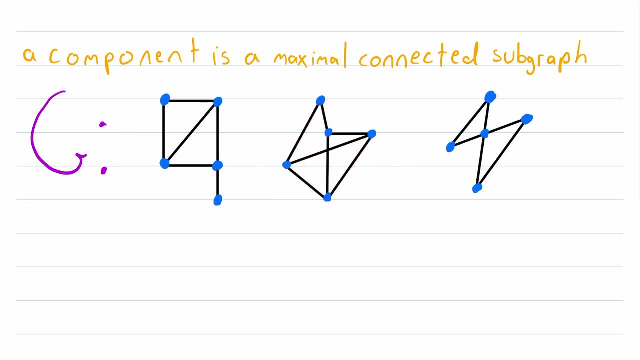 preserving connectedness. And, of course, the same thing is true about this whole sub graph over here. This is another component of G because it is a maximal connected sub graph. Now, before we go, let's go over just some slightly weirder examples. If this was the entirety of the graph G, 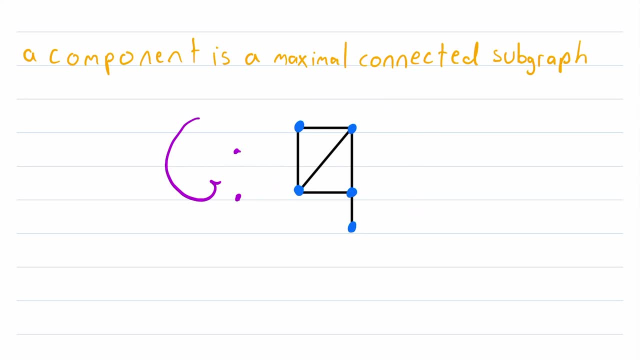 then this would still be a component of G. G has only one component in this case, So sometimes the entire graph is the only component. As you might realize, this is the case with any connected graph. a connected graph has exactly one component. 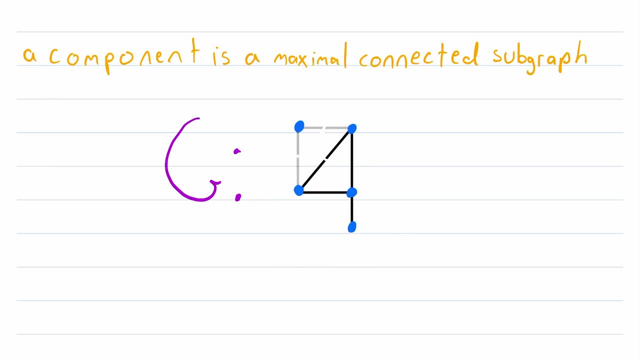 which is the entire graph itself. Also another example that might make you a little uncomfortable: a single isolated vertex is also a component. So if this is our graph G, this has two components. The isolated vertex is one maximal connected sub graph And then this: 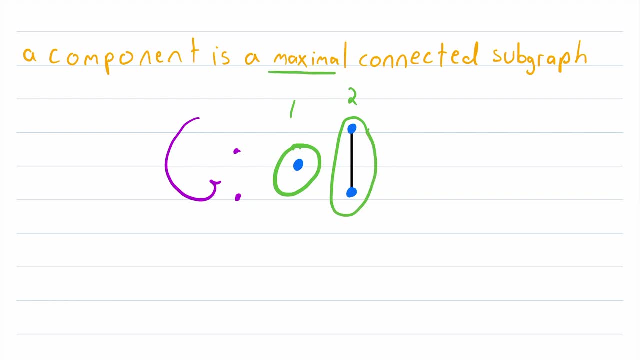 complete sub graph on two vertices is another maximal connected sub graph. So that is what a component of a graph is. I think the simplest way to think about it is that a component of a graph is a sub graph that cannot be extended while preserving connectedness by including.